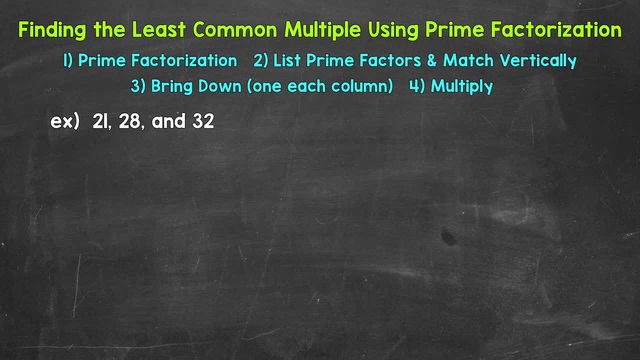 Let's jump into our example where we have 21,, 28, and 32.. So we need to find the least common multiple. Let's find the least common multiple. So we need to find the least common multiple of those three numbers. Let's start with the prime factorization of all three of our numbers. 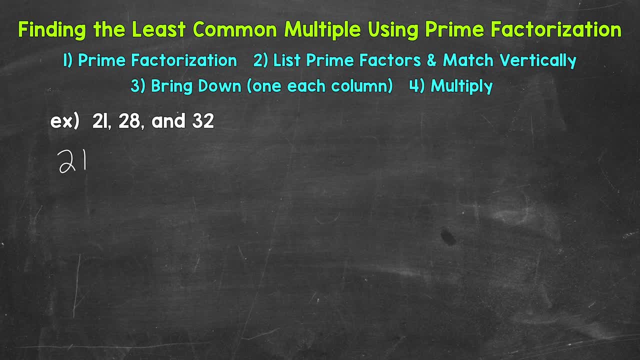 starting with 21.. 3 times 7 equals 21. So 3 and 7 are factors of 21.. Now, 3 is prime, so we are done there. 7 is prime as well, so we are done there, And that's the prime factorization. 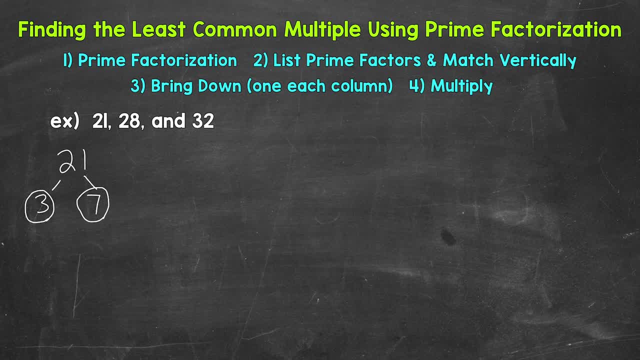 of 21.. We can't break that down any further. Let's move on to 28.. 2 times 14 equals 28.. So 2 and 14 are factors of 28.. 2 is prime. so we are done there. 14, we can break down 2 times 7, equals 14.. So 2. 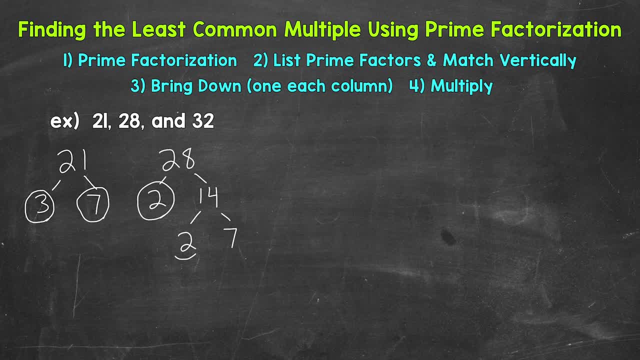 and 7 are factors of 14.. 2 is prime, So we are done there. 7 is prime as well, so we are done there, And that's the prime factorization of 28.. We can't break that down any further. Lastly, we have the prime factorization of 32.. 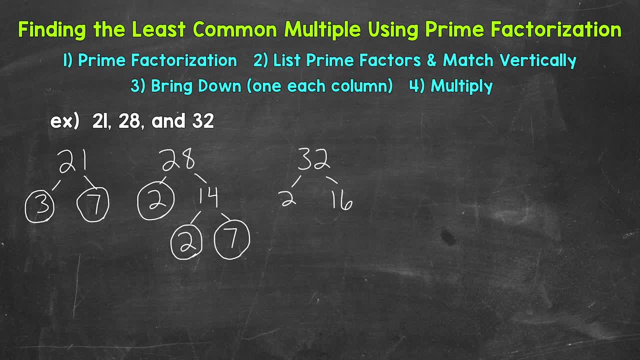 2 times 16 equals 32.. So 2 and 16 are factors of 32.. 2 is prime, so we are done there. 16, we can break down 2 times 8, equals 16.. So 2 and 8 are factors of 16.. 2 is prime, so we are done there. 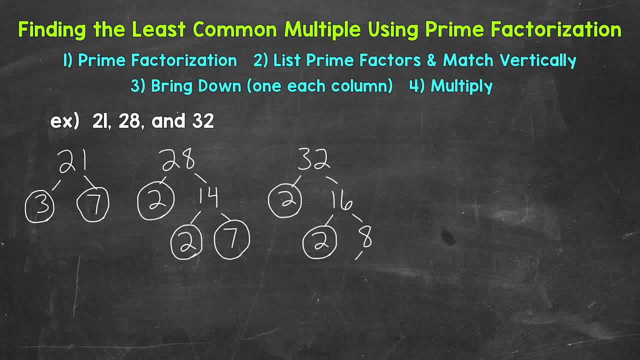 We can break 8 down further 2 times 4 equals 8.. So 2 and 4 are factors of 8.. 2 is prime. so we are done there. We can break 4 down further 2 times 2 equals 4.. So 2 and 4 are factors of 8.. 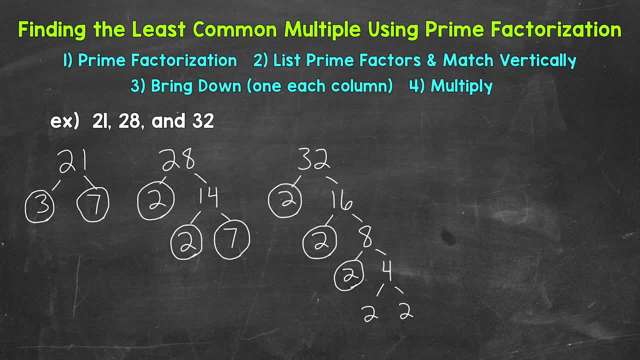 2, times 2 equals 4, so 2 is a factor of 4.. 2 is prime. so we are done there and there, And that's the prime factorization of 32.. We can't break that down any further. 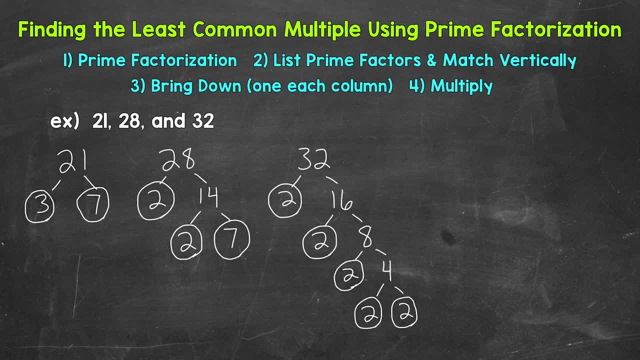 Now that we have the prime factorization of all three of our numbers, we need to list the prime factors and match them vertically. Let's start with the prime factors of 21,. so 3 and 7.. 3 times 7 equals 21.. 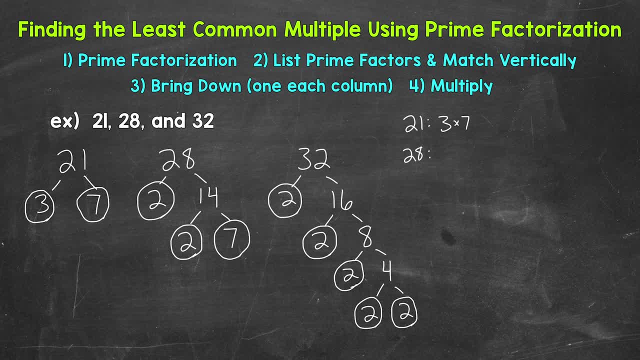 Now for the prime factors of 28,, and I'm going to start with the prime factor of 7.. Since 21 also has a prime factor of 7, I'm matching the 7s vertically. Then we have 2 and 2.. 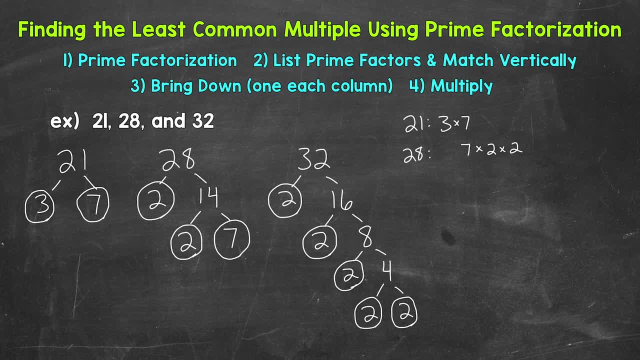 So 7 is a prime factor of 7, and there, 7 times 2 times 2 equals 28.. And then, lastly, we have the prime factors of 32.. We have a 2 that we can match vertically, another 2 that we can match vertically. 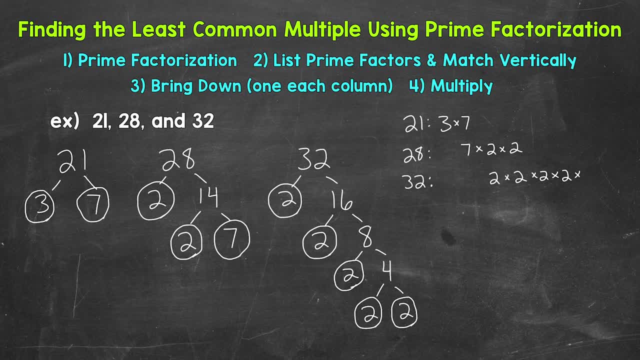 and then three more 2s. Now that we have our prime factors listed and matched vertically, we need to bring down a number to represent each column, And it's going to be 1. 1 for each column. You'll see what this means as we go through this step. 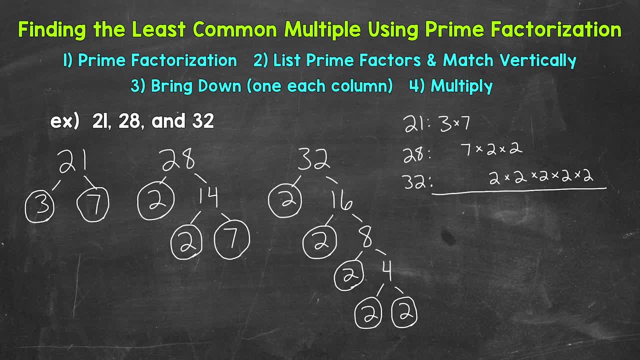 So I like to draw a line to separate our steps here And now again, we need to go through each column and bring down a number to represent that column. For example, we have a 3 column right here, Even though there's one 3, that's okay. 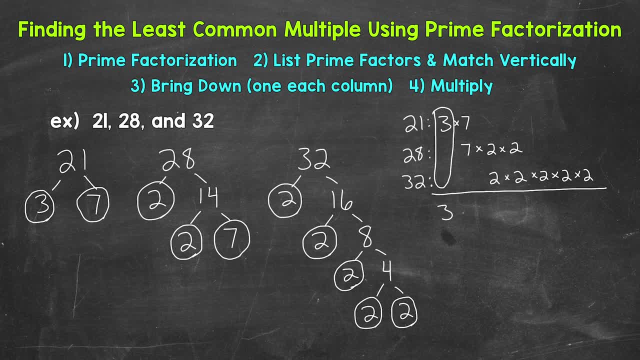 We have a 3 column there, So let's bring down a 3 to represent that column Times. We have a 7 column here. Now there are two 7s there, but we only bring down one 7 to represent that column. 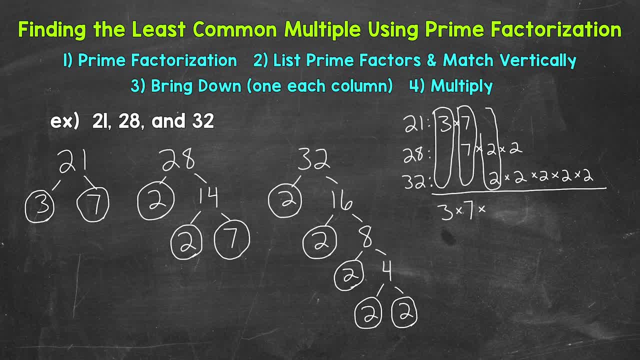 Times. Next, we have a column of 2s, So bring down a 2 to represent that column. And then another column of 2s, So bring down another 2 to represent that column Times. We have one 2 here, but it is a column. 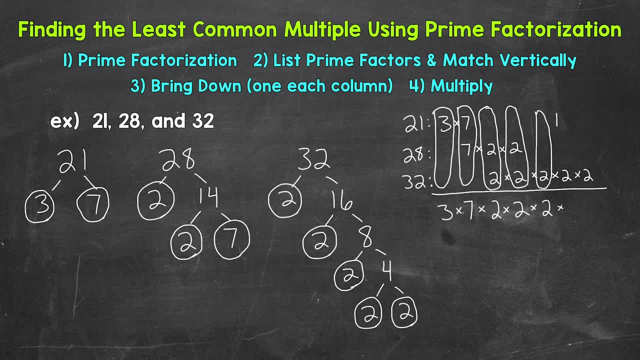 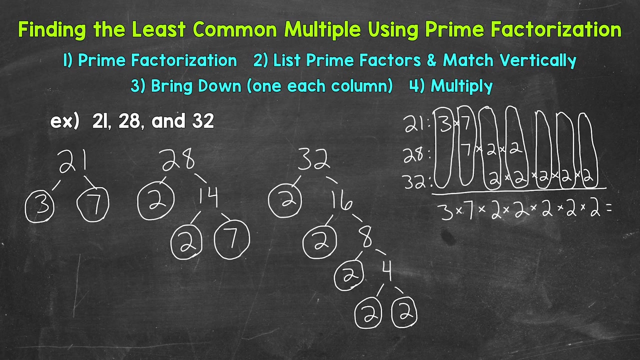 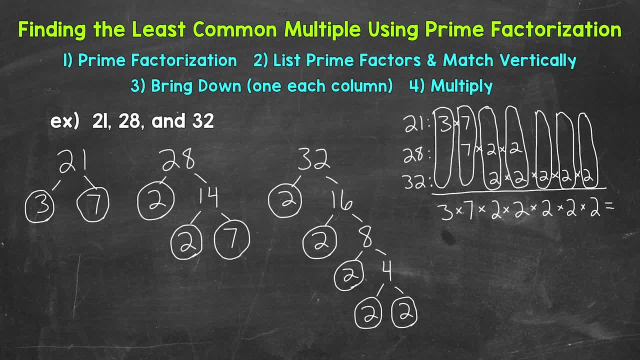 Now there are different ways to go about multiplying these numbers. For example, you can start with 3 times 7 and work your way from left to right. I'm going to start with this group of 5 2s right here. So we 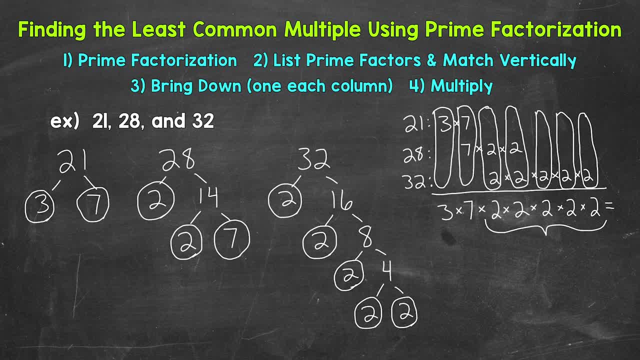 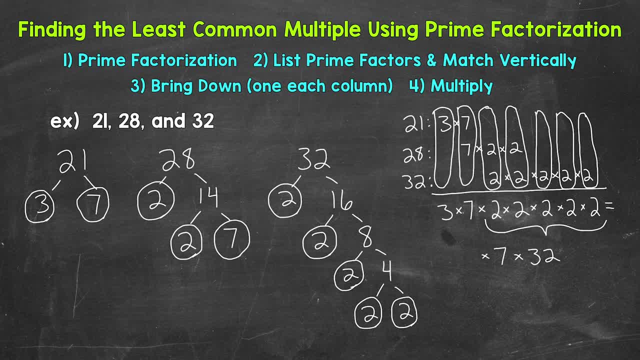 can bring down our 7 and 3.. Now again, there are different ways to go about multiplying these numbers. I'm just going to work from left to right, So I'll do 3 times 7 next, which is 21.. 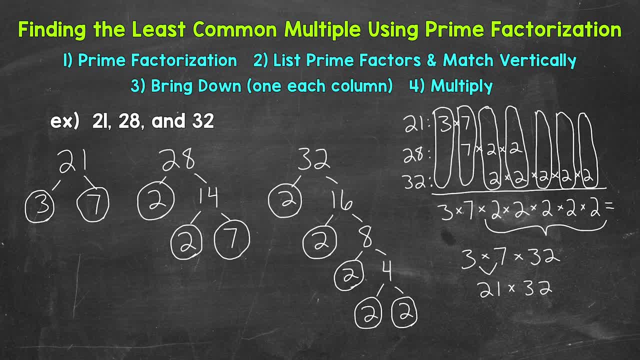 And then we have 21 times 2 times 2 times 2.. 21 times 32 for our last step. Now I'm not sure what 21 times 32 is, so I need to work this out off to the side. So 32 times 21.. I put the larger number in value on top. Let's. 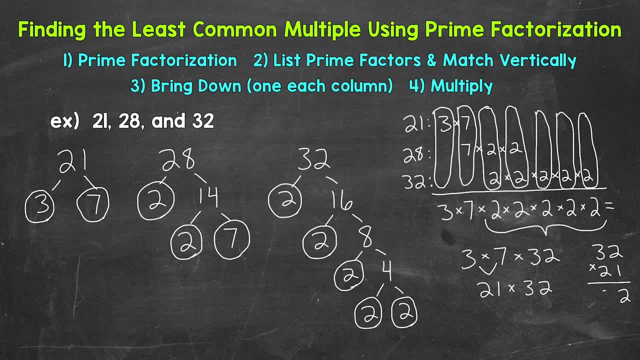 multiply 1 times 2 is 2.. 1 times 3 is 3.. We are done with this: 1.. And now we need that 0.. 2 times 2.. 1 times 2 is 4.. And then 2 times 3 is 6.. Now we add 32 plus 640.. 2 plus 0 is 2.. 3 plus. 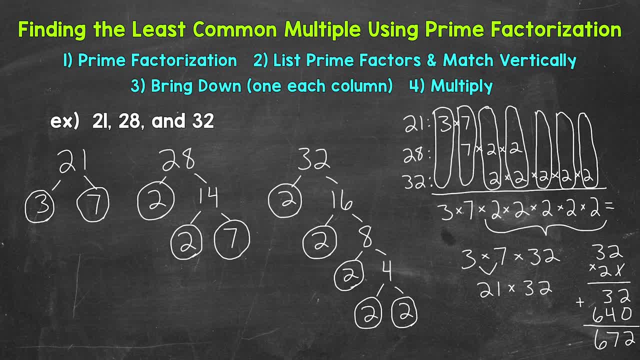